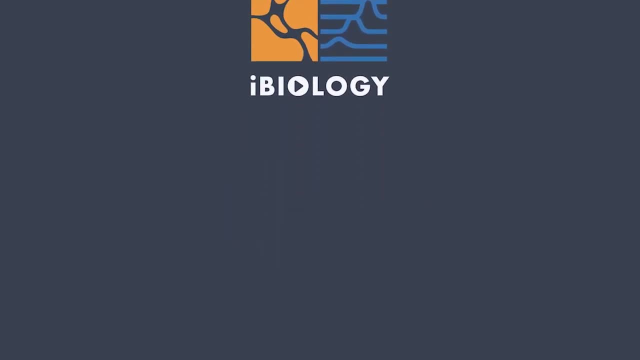 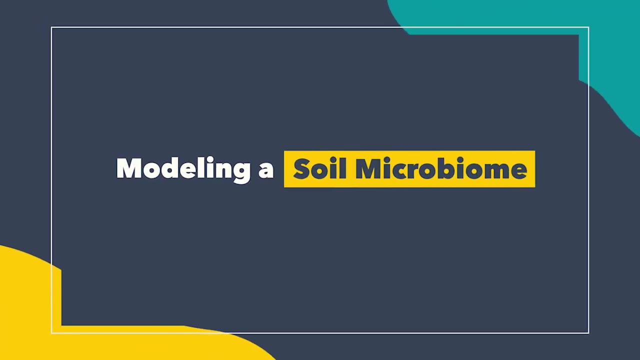 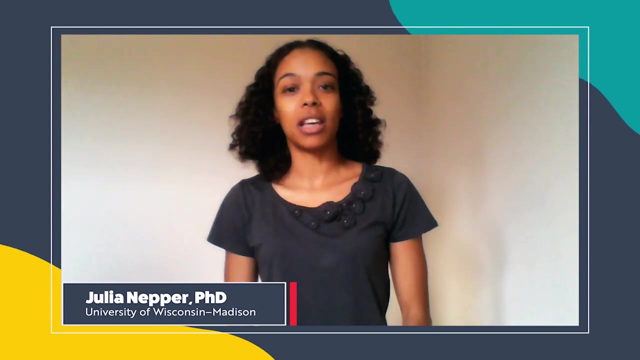 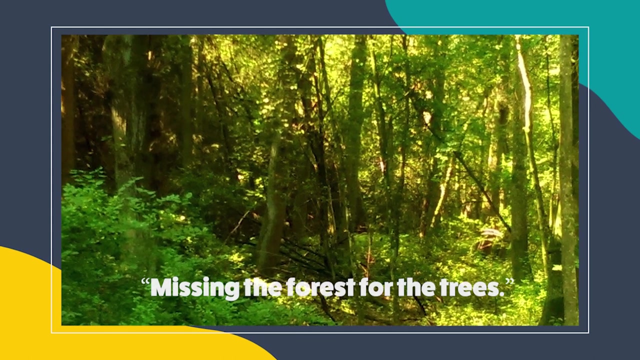 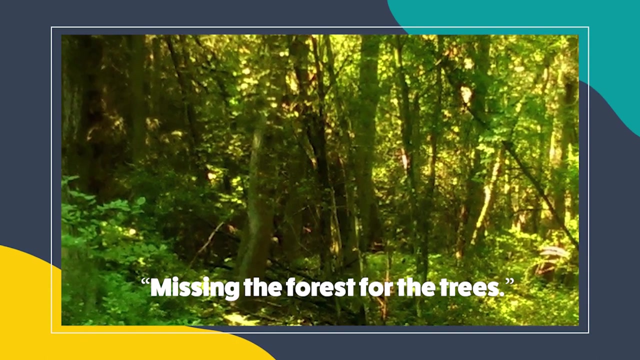 Hi, my name is Dr Julia Knepper, and today I'm going to be telling you about how to model a soil microbiome. So I want you to think of the adage missing the forest for the trees. If you're not familiar with this saying, what it means is that you're focusing so intently on one particular. 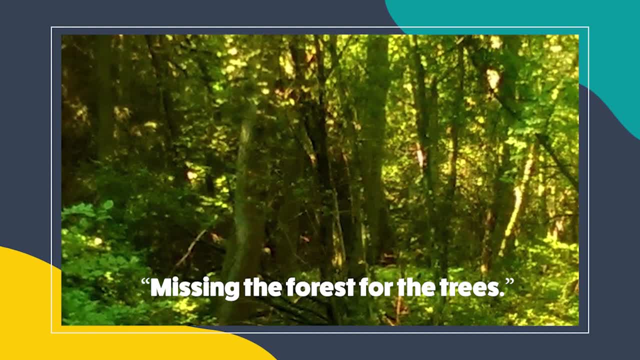 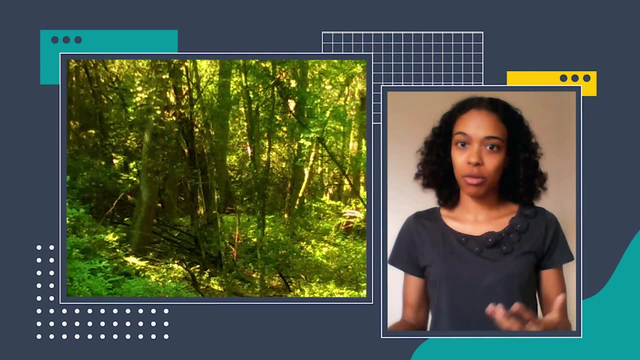 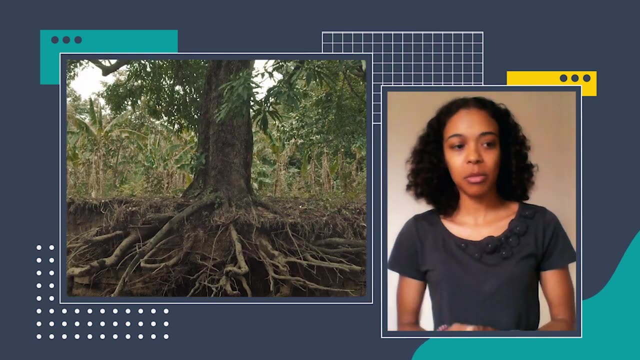 aspect of something that you're missing: the larger context. Now, I don't study trees, I study soil bacteria, but the underlying principle of understanding the larger context is part of what I study. There's another thing that you may not think of when you think about trees, and that's 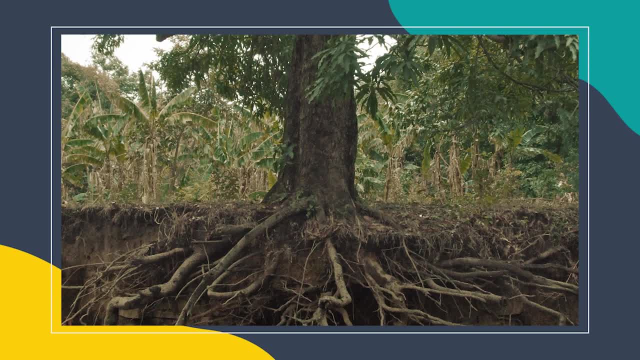 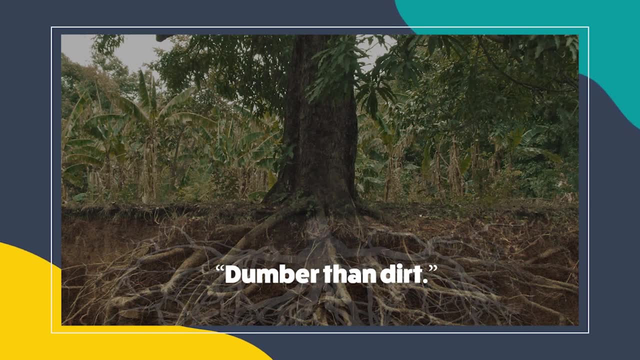 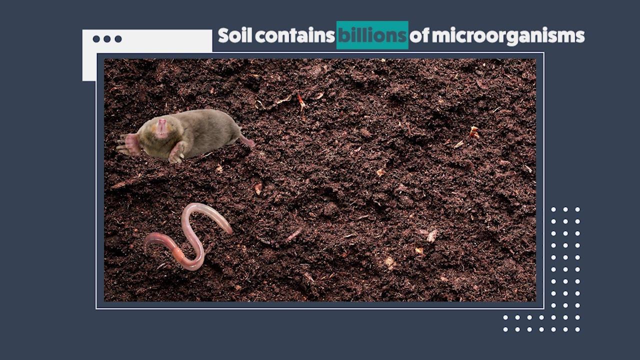 the soil and the roots. and there's another saying that's common: dumber than dirt, and I'm going to show you today that soil is anything but stupid. Far from being an inert mass of minerals, soil is actually full of life. There are larger creatures that you may be more familiar with, like moles, and 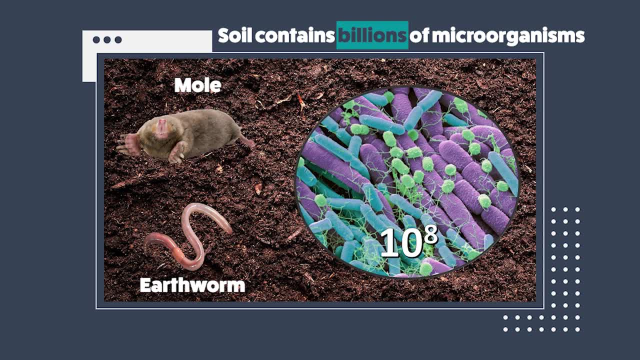 earthworms, but in addition there are billions and billions of microorganisms. A single teaspoon of rich soil can have as many microorganisms, as many bacteria, as there are people in the United States. So hundreds of millions of bacteria per teaspoon. So what we're interested in doing with 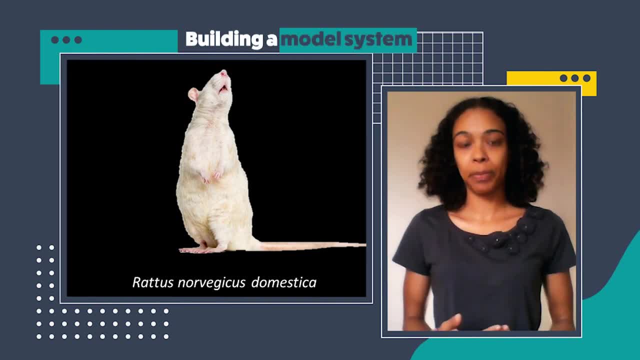 these bacteria is forming what's called a model system. Model systems are very useful tools for simplifying a problem and taking it to the lab and doing experiments with it that we can then extrapolate to a different, more complex model. So what we're going to do is we're going to take 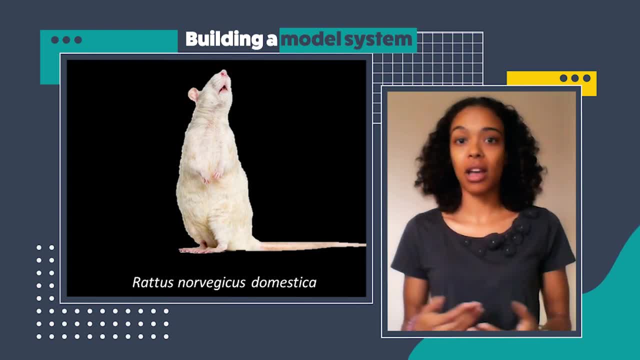 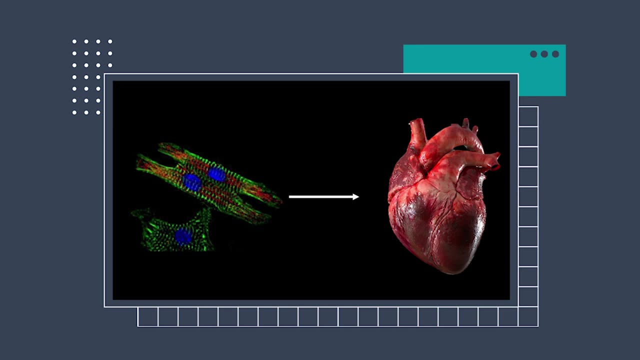 a complex system. One that you may be familiar with is the common lab rat, Rattus norregicus domestica, which we use as a model for understanding diseases in humans, as well as understanding rats, And one of the reasons why we're interested in this is because we can often find emergent 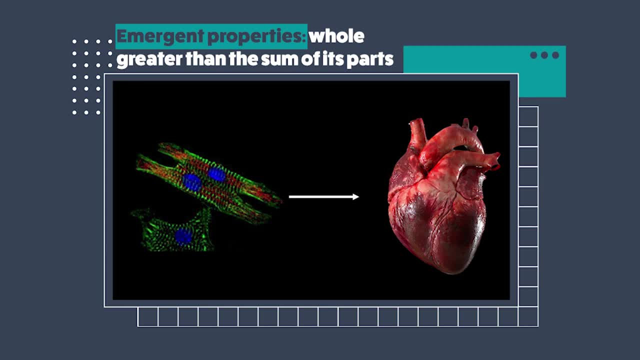 properties when we look at systems in their entirety. So what this means basically is that the individuals together are greater than the sum of their parts. So you can think of, for example, a heart. Heart cells individually are not able to pump blood through our body. 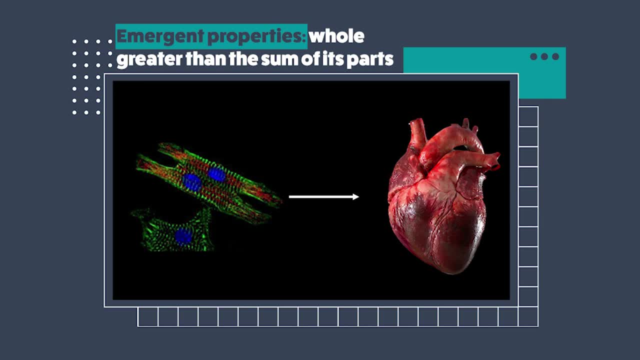 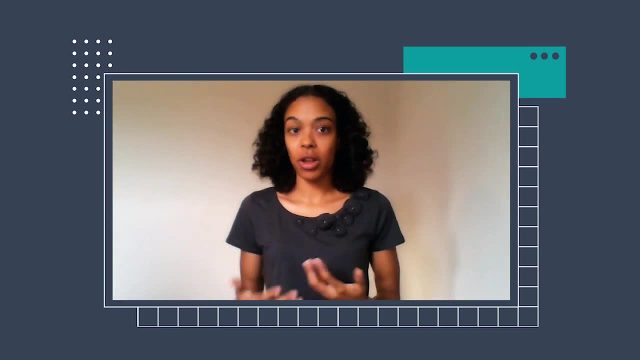 but if you get billions of them together, then you can form the organ, the heart, which has the emergent property of being able to pump blood. Now I told you that I was going to talk about soil bacteria, but even that is a bit too large of a problem to tackle with just one model. 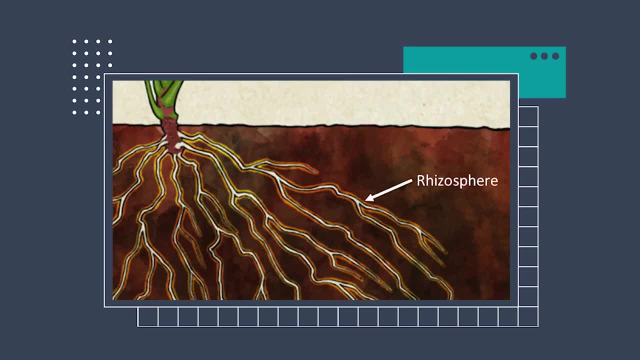 But what I'm actually going to be talking about today is a zone specifically called the rhizosphere, from the Greek rhizo meaning root. You can think of this as the plant-root microbiome. It's basically the area of soil directly on and about a millimeter away from the roots, and this is the area of soil. 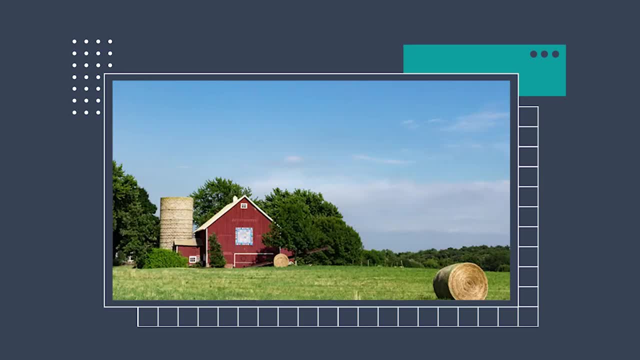 that's directly impacted by plants. One of the reasons why we're very interested in the rhizosphere is because of agricultural reasons. If we can directly affect the rhizosphere, then we can have effects on the plant that can cause them to be more drought resistant or to produce more fruit. 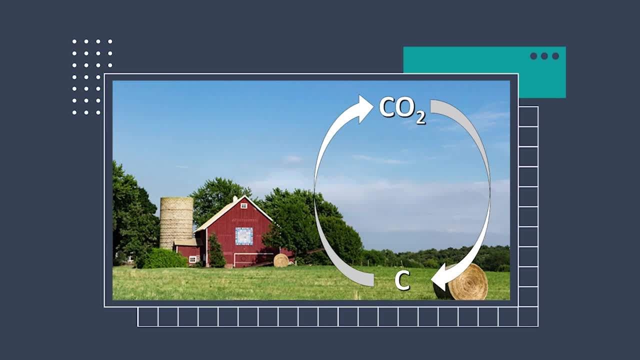 etc. Another reason why we're interested in studying the rhizosphere is because it can affect plants' ability to take up carbon dioxide and form it into other carbon compounds which it uses to build itself. So if we can somehow alter the rhizosphere so that the plants are better, 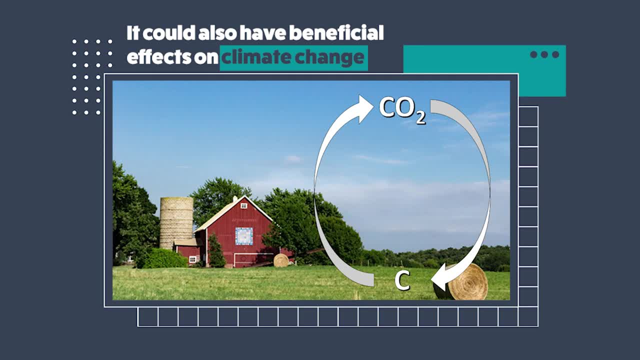 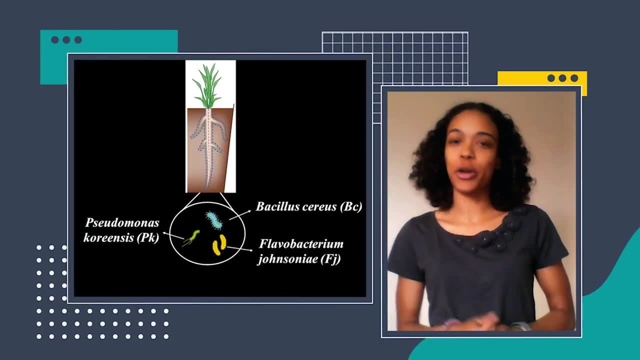 able to take up carbon dioxide, then it's possible that we could have some beneficial effect on climate change. So I'm going to spoil a punchline a little bit and I'm going to tell you what the model system is before I tell you how we got there. It's called THOR, Not the one you're. 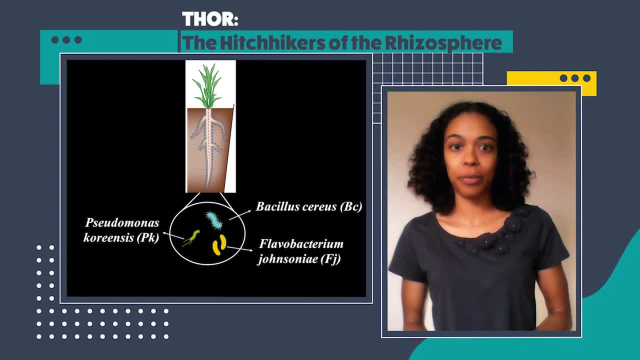 thinking of. It stands for the Hitchhikers of the Rhizosphere, And it's a model system composed of three different bacteria: Pseudomonas coriensis, Flavobacterium johnsonii and Bacillus cereus, which I will refer to as PK, FJ and BC. So the first question, of course, 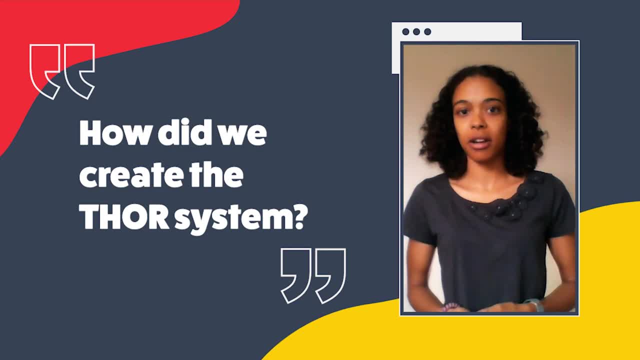 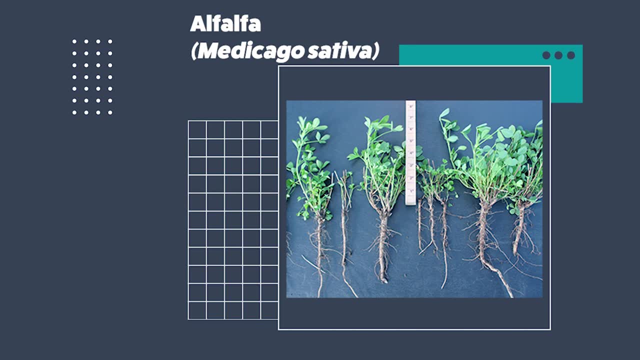 is: how did we create this system? How did we get here? Well, this started with some agricultural research, in fact about 30 years ago, where researchers were trying to find biological agents that could control disease. So the first thing they did was they looked at a bunch of different species of alfalfa. as opposed 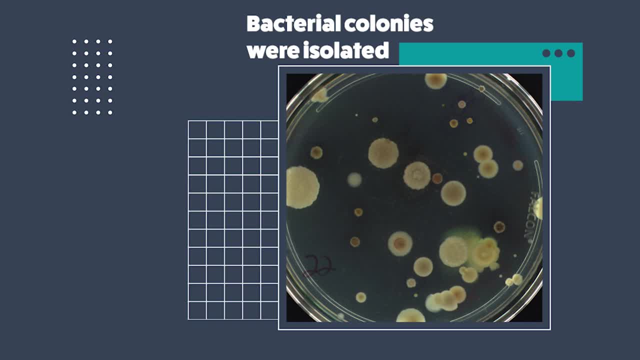 to chemical agents like pesticides. The way they went about this is by isolating bacteria directly from the roots of the alfalfa plants. You can see the results of an example: isolation from roots. We get all of these individual colonies, which are themselves propagations of an individual species. 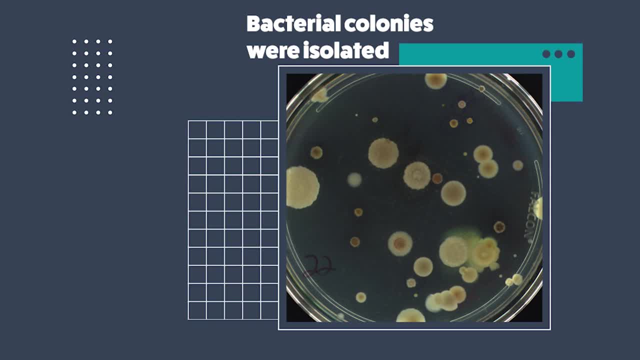 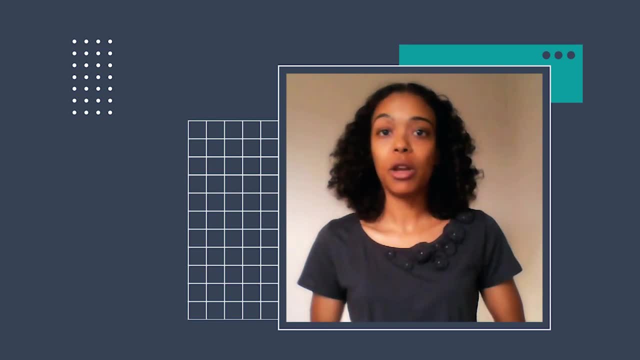 or strain of a species. So then we can select those colonies from the roots of the alfalfa plants and then we can look at the results of that analysis. So the researchers isolated 700 different bacteria from the roots of alfalfa. They only found one. 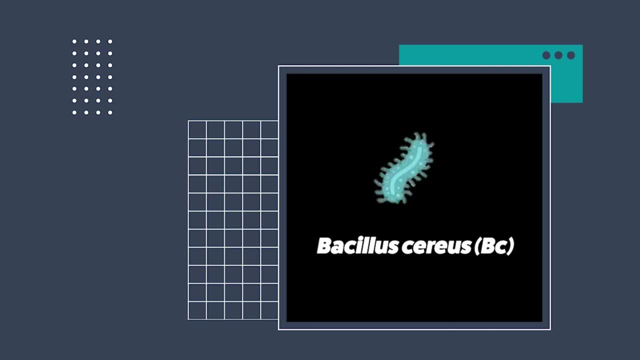 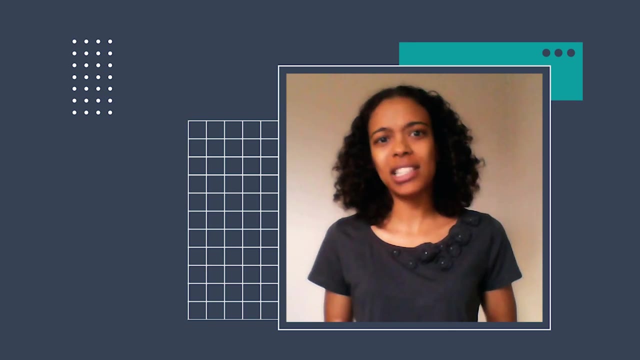 that was able to prevent the disease that they were looking at and that was BC. But there was an issue when they actually took it back to the field and tried to apply BC to fields of alfalfa to prevent this disease, And that was that it was only somewhat effective, sporadically effective. 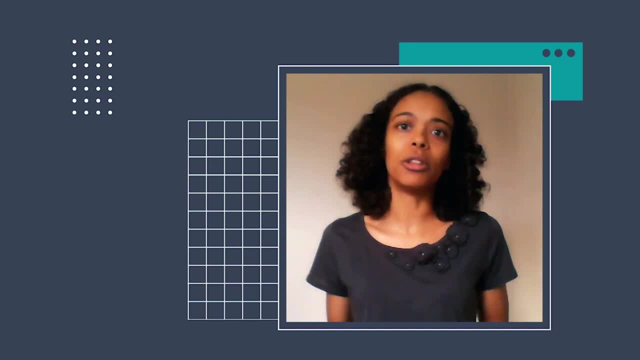 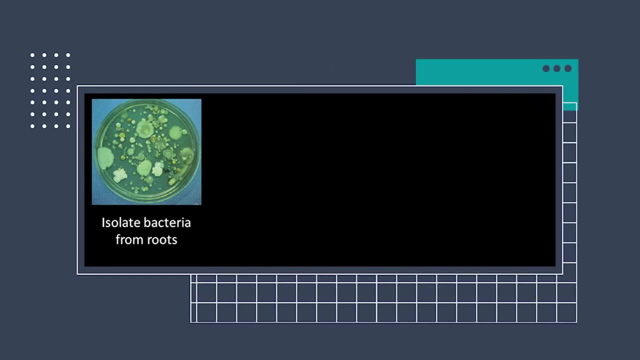 and so they decided: well, let's look at what the larger context is of what this BC is existing in. So one thing that's really interesting about BC is that it carries what's called biological hitchhikers. We're not exactly sure why it does this, but it could be because these bacteria are 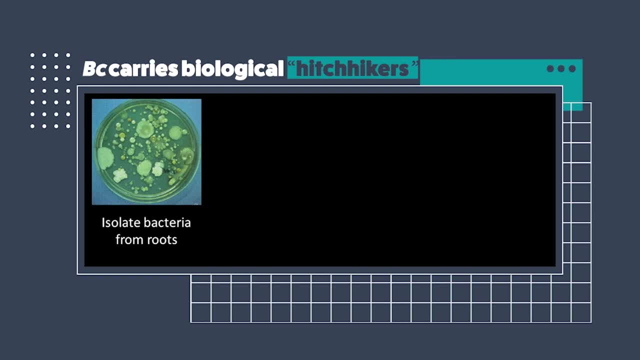 using BC to get somewhere, or using it for nutrients or something like that. So, basically, what a hitchhiker is is you will isolate the bacteria from roots, as before, And then you will take the individual colony that you're interested in and you will attempt to purify it. So you'll passage. 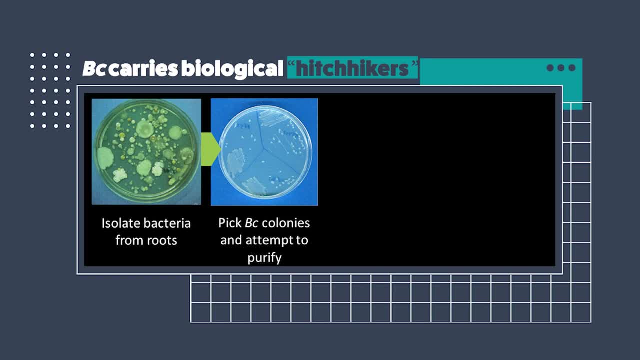 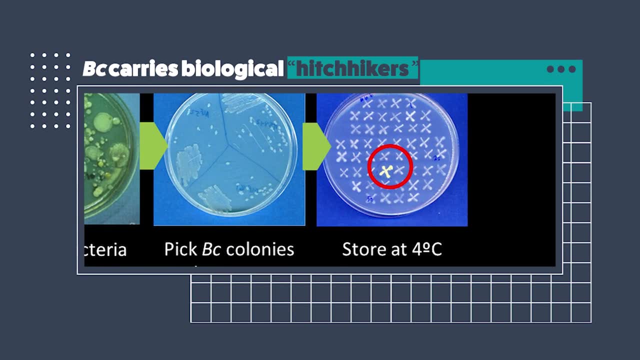 it on media a bunch of times until it looks like you just have that one particular bacterium And then you put it at the fridge for a couple days and you come back to it and suddenly there's a new species there, There's a. 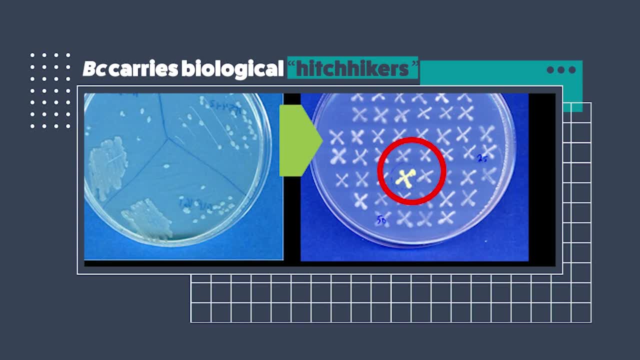 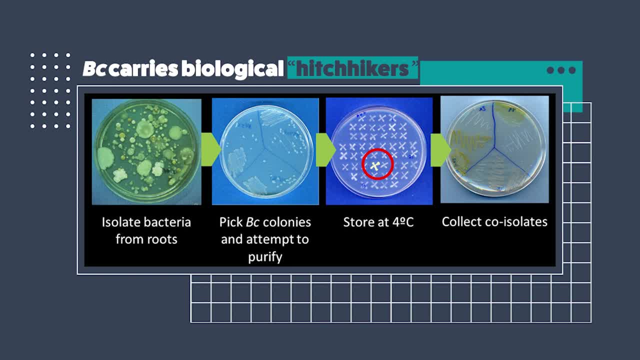 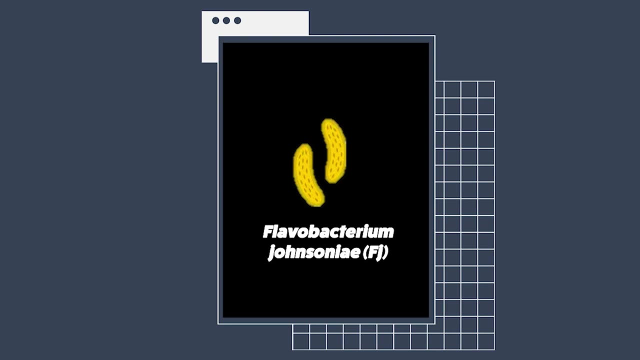 So then we can take that species and we can re-isolate the BC and isolate the new species and we can start to characterize both of them. One hitchhiker that's very common on BC is FJ, And it seems that the reason for this is because FJ actually uses BC to be able to survive in the 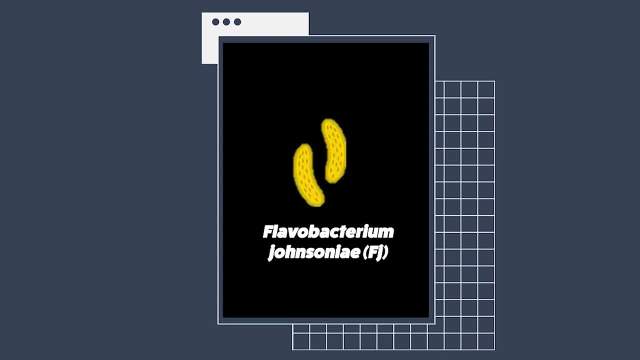 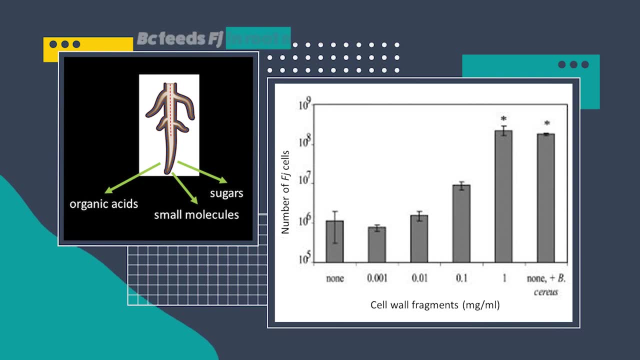 rhizosphere. So to imitate the rhizosphere environment in the lab we use what's called root exudate medium. So plants secrete a lot of molecules from their roots all the time, and root exudate is composed of things like sugars, organic acids and other small molecules. 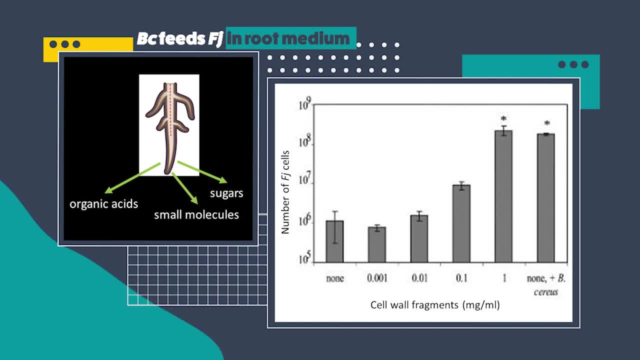 So we take that and we make it into a medium in which the bacteria can grow. BC grows just fine in this medium, but FJ does not. So in the graph on the right, on the vertical y-axis, what we're looking at is the number. 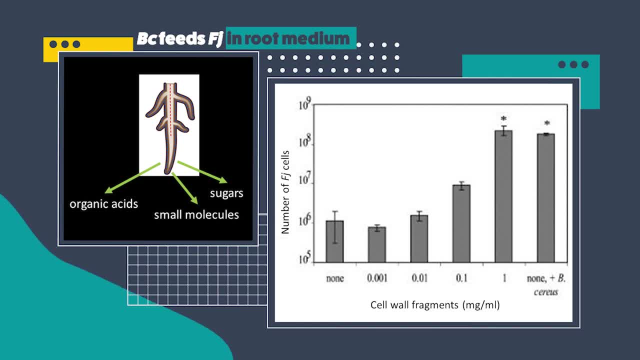 of FJ cells And on the horizontal x-axis we have different concentrations of cell wall fragments. So BC will actually shed parts of its cell wall into the medium and this is what actually feeds FJ. So you can see that as we get higher concentrations of cell wall fragments or on the rightmost, 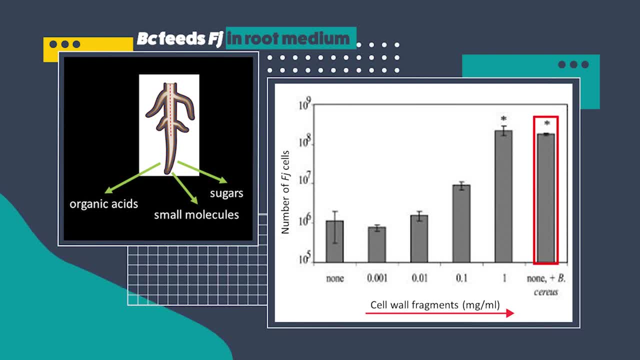 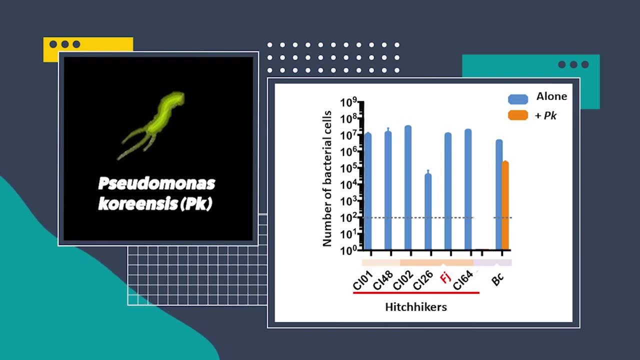 bar. if we simply add BC, then FJ is suddenly able to grow in this medium, indicating that it's the cell wall fragments that are feeding FJ in this medium. There's another hitchhiker that's of particular interest to us in the lab, and that's PK. 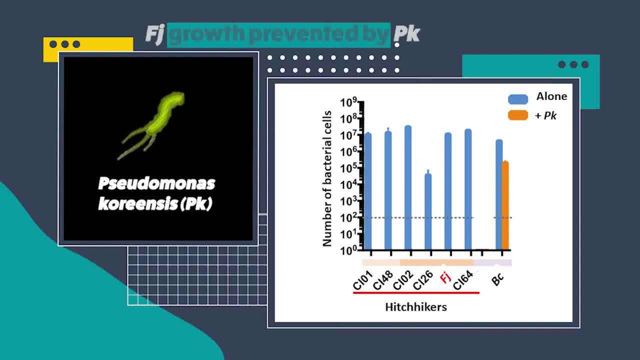 Interestingly enough, PK actually inhibits the growth of FJ And other co-isolates that are closely related to it. So in this graph, again on the vertical y-axis, we have number of bacterial cells, And that's not just of FJ, it's of whichever isolate is labeled on the bottom. 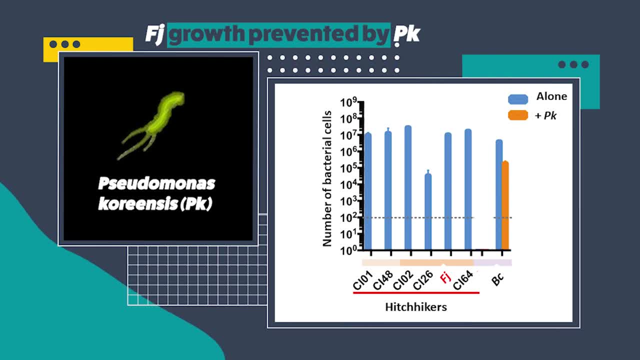 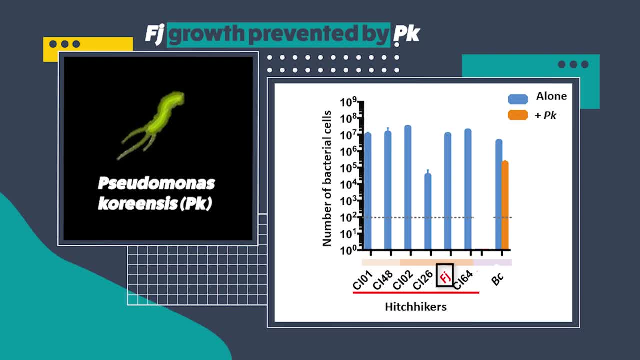 So the blue bars are showing the amount of growth that you get with these isolates when they're in isolation, And then the orange bars are showing the amount of growth that you get when you add PK. You'll see that there aren't any orange bars, except in the case of BC, because PK actually 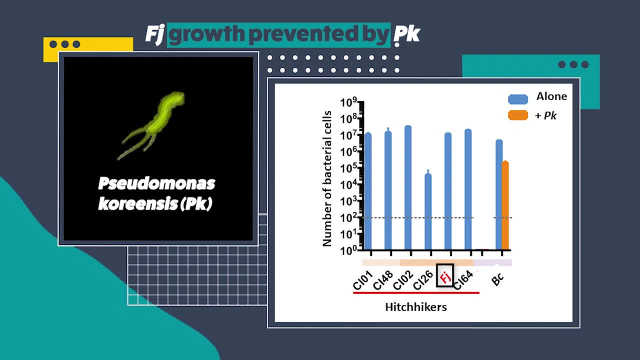 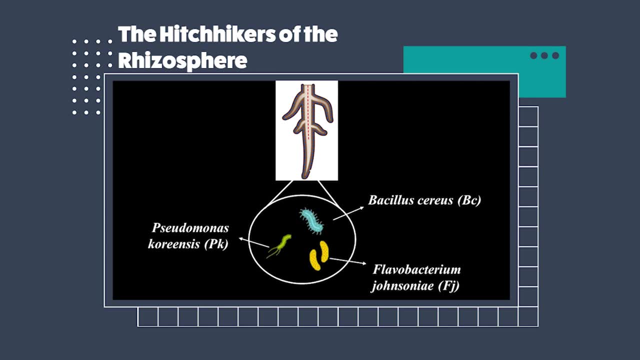 kills all of FJ and it's closely related co-isolates. So it was clear to us that these three species were the ones that were the most likely to kill FJ. So it was clear to us that these three species were the ones that were the most likely to. 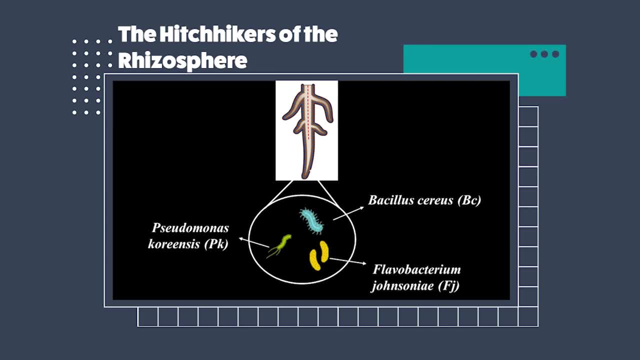 kill FJ. So it was clear to us that these three species were the ones that were the most likely to kill FJ And that these three species were interacting in nature, and interacting in interesting ways that you wouldn't expect if they were just strangers in the night passing each other. 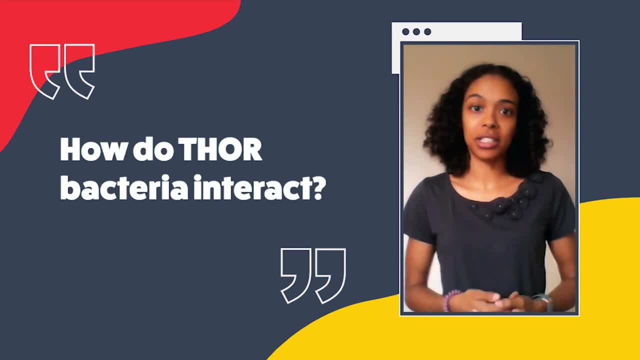 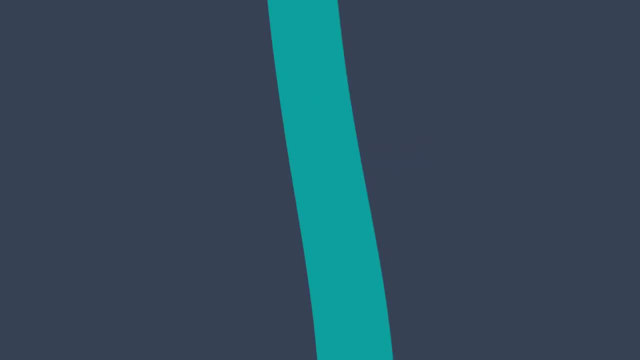 So the next question that we wanted to ask after we established this system is: how do these bacteria interact? We need to characterize our system so that we can use it better. So one of the first things that we noticed is that BC actually prevents PK from killing. 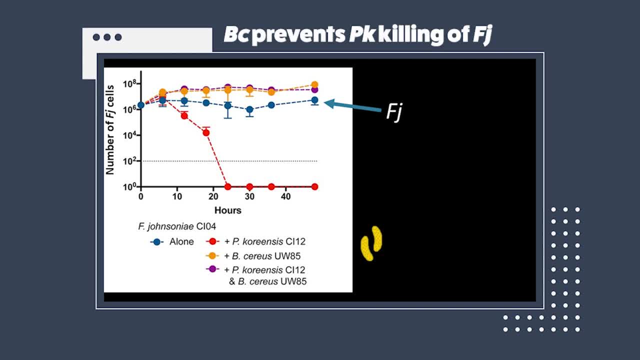 FJ. So when we grow FJ in isolation in the blue line again it reaches a certain level, as you can see on the vertical y-axis, which is indicating the number of cells of FJ. But if we add PK in the red line then you can see that over time, as indicated on the 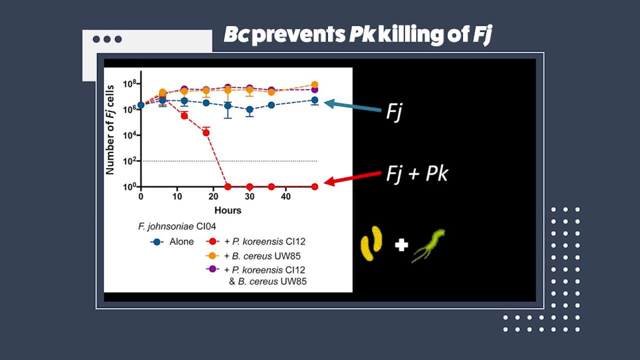 horizontal x-axis PK will completely kill all of the FJ until FJ is no longer detectable. But if we add BC to this mixture, the full three-member community in one tube- then FJ is able to grow just fine perhaps. 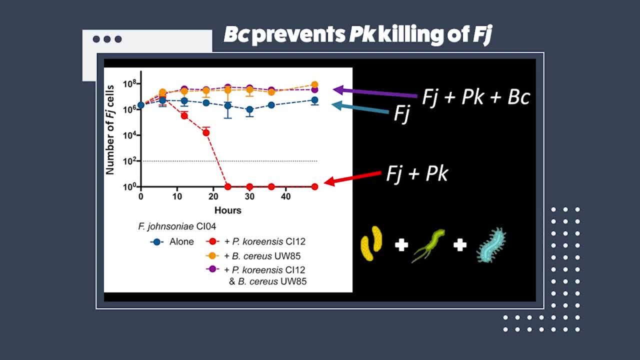 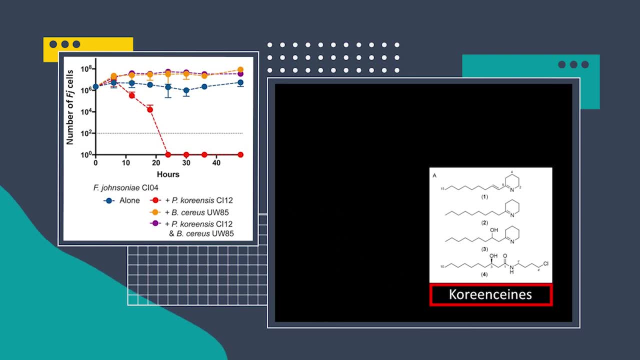 even slightly better than it would grow on its own. And we found that the reason for this is an antibiotic set of molecules called coriancins that are actually produced by PK in response to the presence of FJ. But when we add BC, then BC prevents the production of these coriancins by PK, allowing FJ to 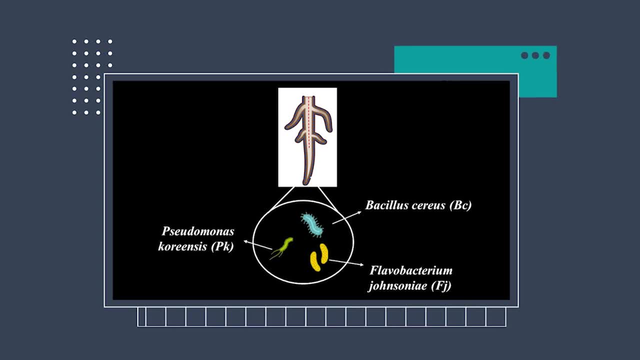 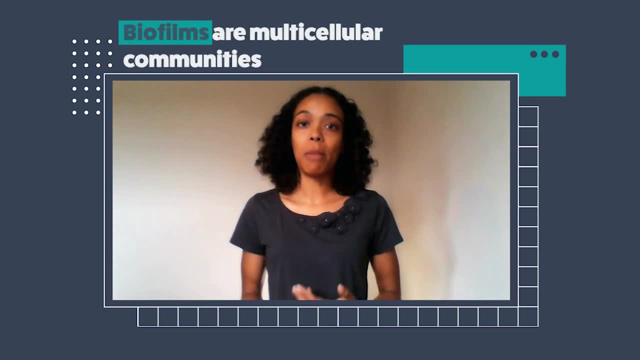 live. There's another really interesting phenomenon that occurs with the three-member community and that's in biofilm formation. So biofilms are multicellular communities of unicellular organisms. Something that you may be familiar with that is, a biofilm is rock slime in a pond or lake. 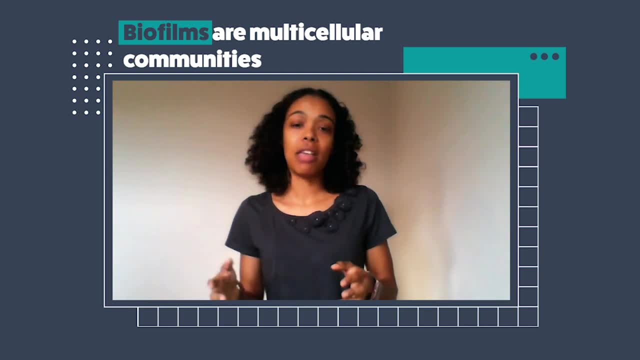 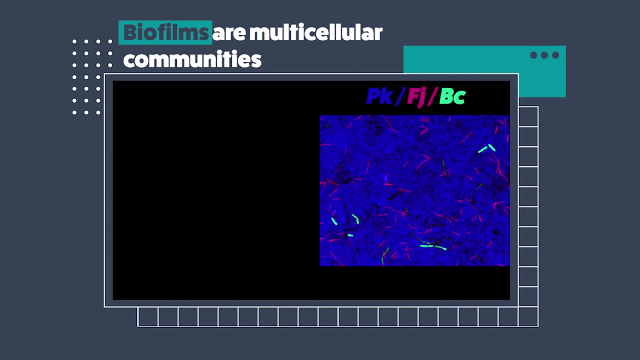 So a biofilm is the cells themselves and then a matrix of sugars and proteins and other molecules That the organisms secrete to keep themselves protected and together. So in the right image you can see a biofilm composed of the three organisms with PK labeled. 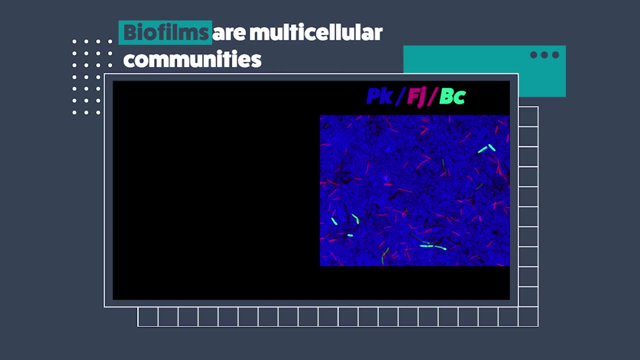 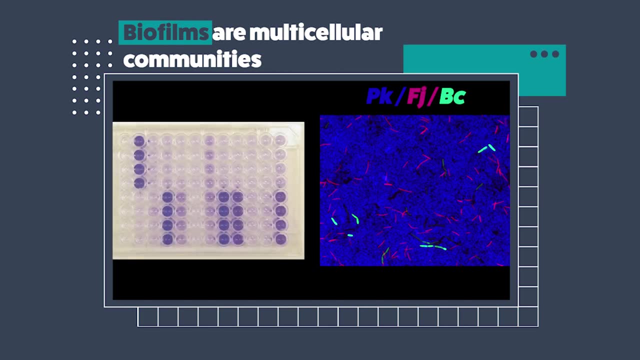 in blue, FJ in red and BC in green, and you can see that they're kind of stably associated with each other. And the way that we measure this in the lab is by growing these cells in what's called a 96-well plate, pictured on the left. 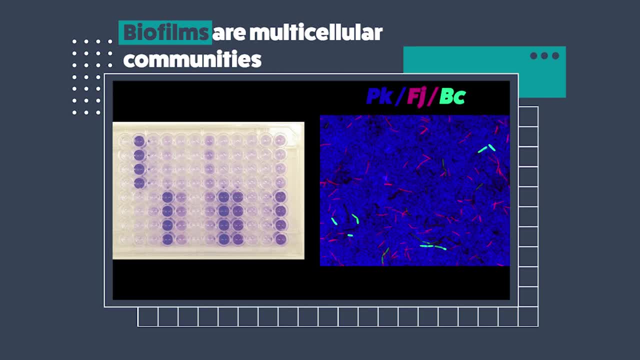 And then, after a certain amount of time, We wash out any cells that are not adhering to the surface and thus presumably not in the biofilm, And then we can stain whatever material remains with what's called crystal violet. And this is like the most exciting part of my week, because most of the things that I 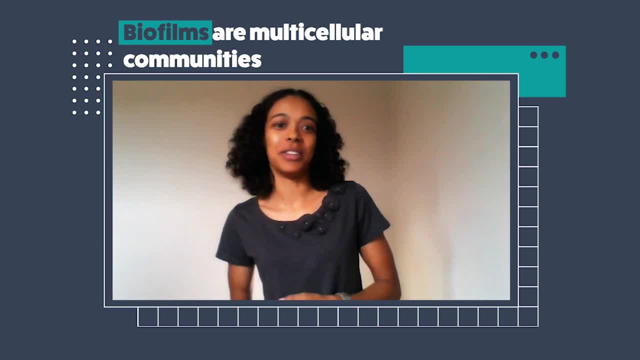 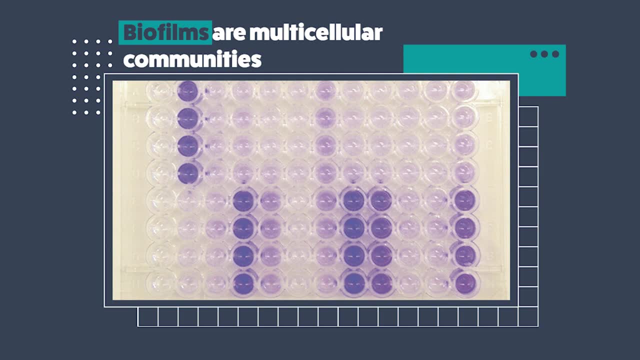 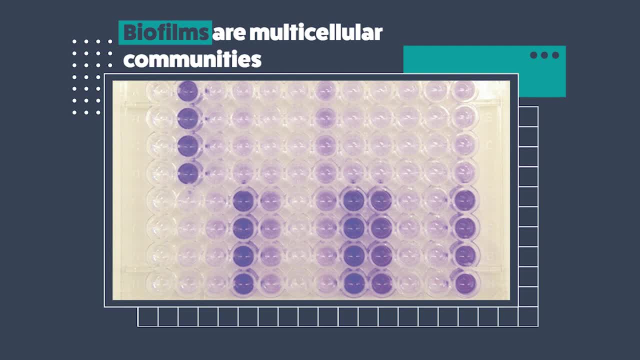 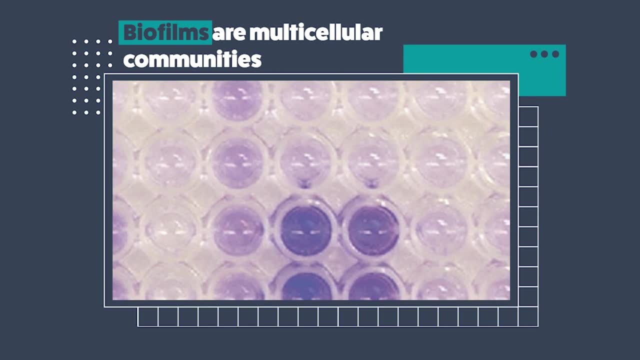 We're ready to go. The purple dye. we can shoot light through each well, and based on how much light passes through, we have an indirect measure of how much biofilm there is. So I was interested in studying this phenomenon when I came to the lab, because I studied biofilms. 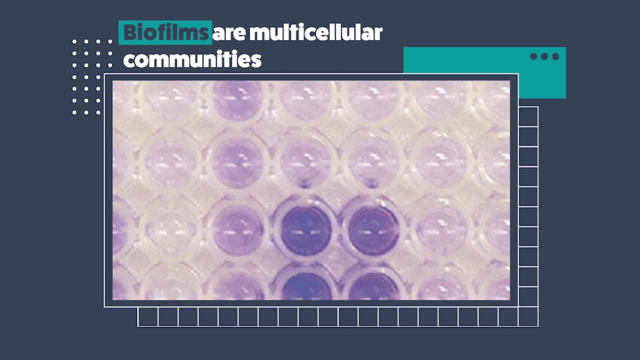 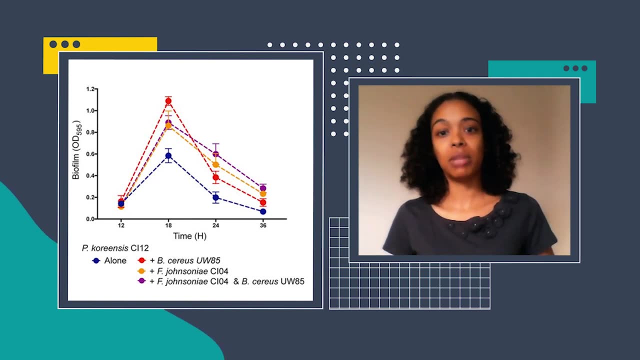 when I was a graduate student, And one thing that we wanted to know is why this was happening. So BC and FJ both cause PK to form more biofilm. So on the vertical y-axis we have measures of biofilm versus time. on the horizontal x-axis, 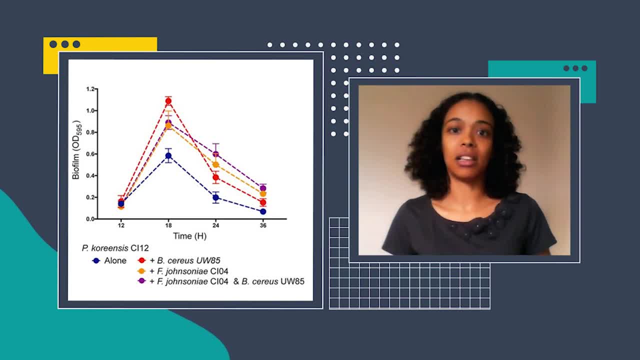 And in the blue line we have just PK itself forming a biofilm. It forms a certain amount and then over time that drops off as the biofilm begins to disperse. Then all of the other lines are PK plus either BC or FJ or both. 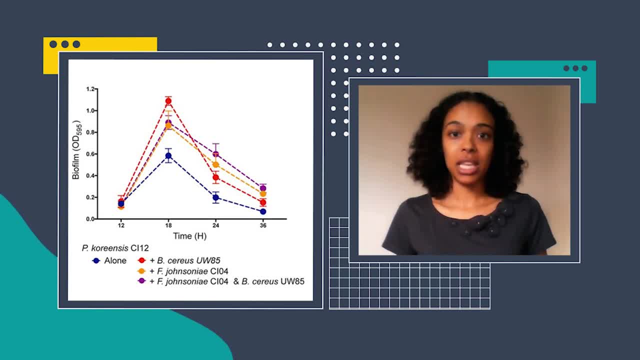 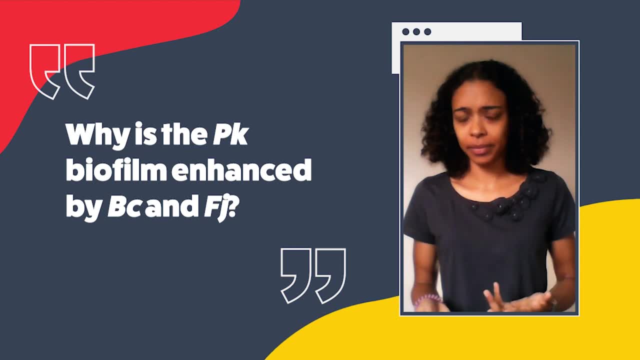 And you can see that in all of these instances there's a difference in the amount of time PK forms more biofilm than it would by itself. So we wanted to understand why is this happening? And at least in the case of BC, it seems to be at least partly because of this other antibiotic. 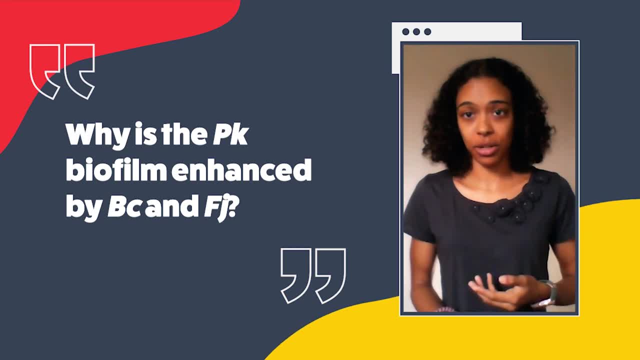 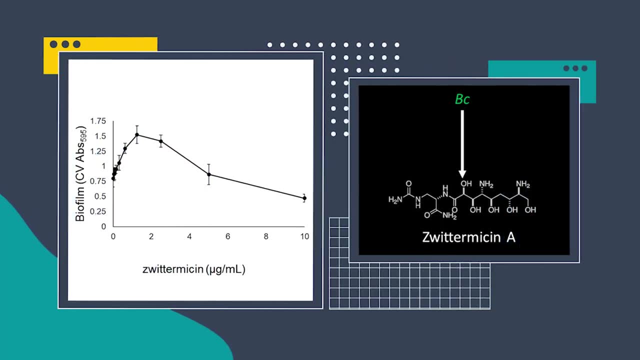 molecule called sweatermycin that BC produces constitutively or all of the time. So we did a simple experiment, We�� PK with differing concentrations of the switermycin, which you can see on the horizontal x-axis, And you can see that when we get a certain concentration of the switermycin then the 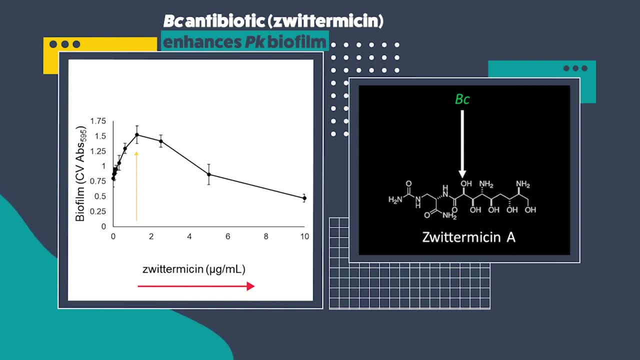 PK biofilm formation almost doubles, as you can see, on the vertical y-axis relative to the level we reach without switermycin, Indicating that perhaps some of theseopia mutations organs to be sound, the surgical implementation of the combination of BNT, fasting, misinformin and FJ can be found on theестоchromicin. 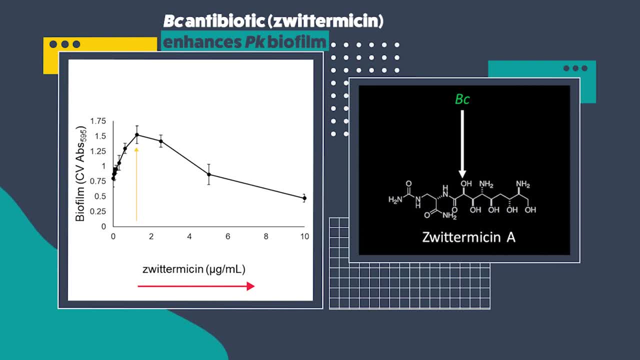 So in 20 minutes we will know when that nel- enthusiasm is gone And we will check our patient of MS Institute. Perhaps sputomycin is not just acting as a killing molecule, as we usually expect for antibiotics, but it may also be acting as a signaling molecule. 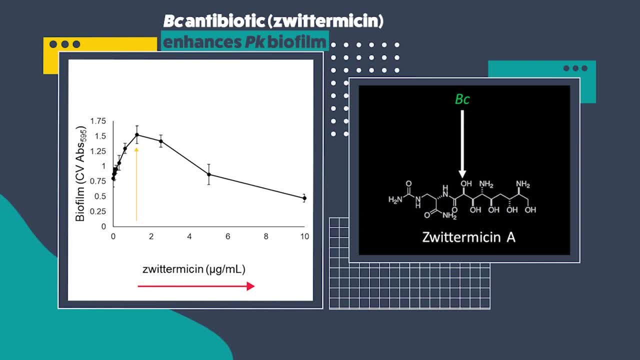 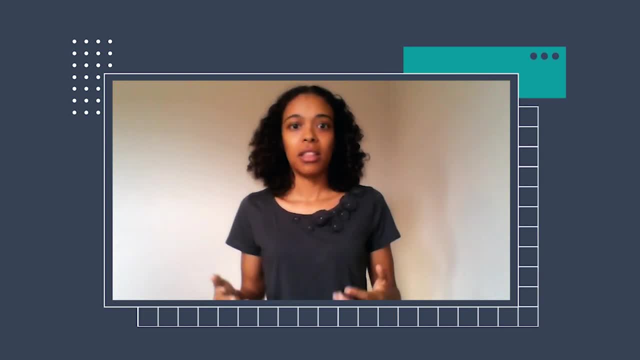 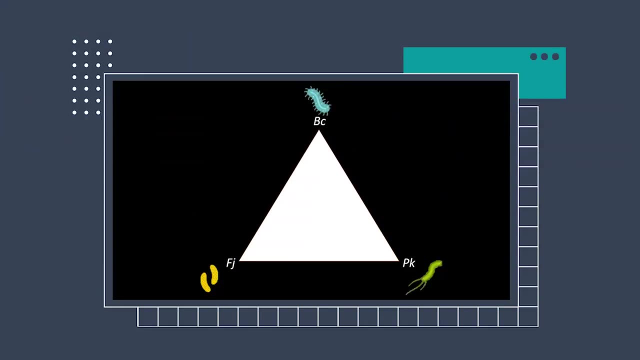 telling PK: hey, I'm around, let's make a biofilm together. So that's the hitchhikers of the rhizosphere, Two bacteria that hitchhike on this agriculturally relevant bacterium, Bacillus cereus. I've shown you that these bacteria 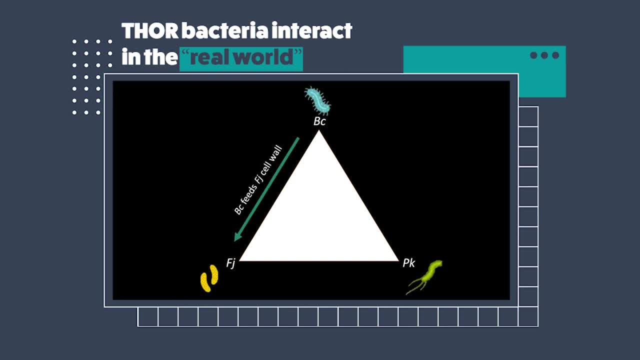 seem to interact in the real world. So BC feeds FJ parts of its cell wall. FJ causes PK to produce coriancins which in turn kill FJ. BC reduces coriancin production by PK, allowing FJ to cohabitate with the other bacteria. 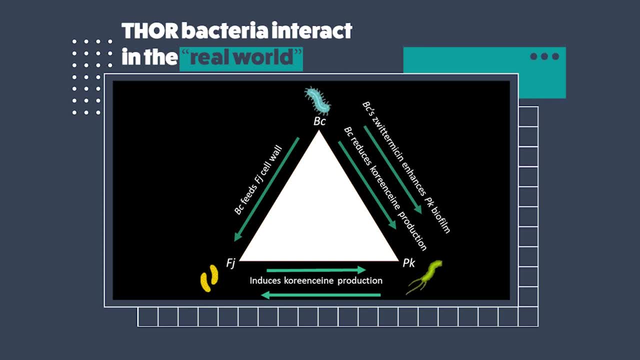 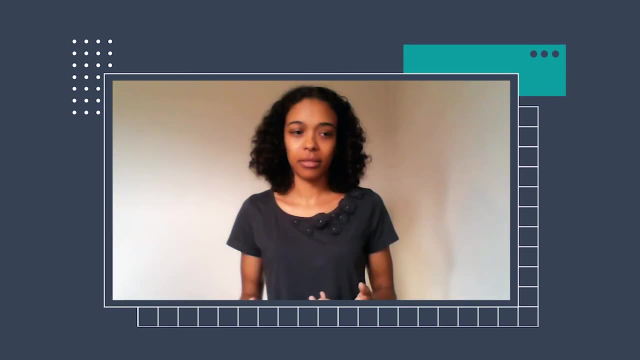 The other two, And the sputomycin produced by BC enhances the biofilm produced by PK, And altogether these three organisms form more biofilm than any of them would on their own. Now, this is a lot to remember, and I don't expect you to remember. 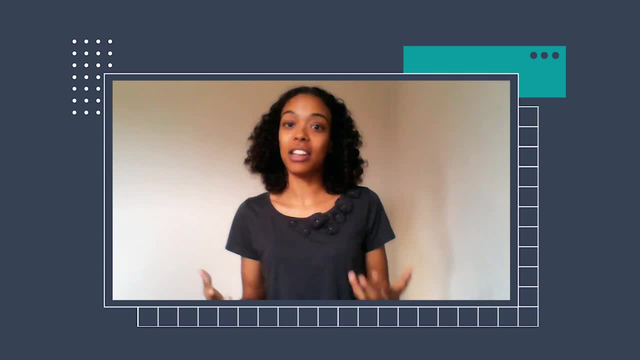 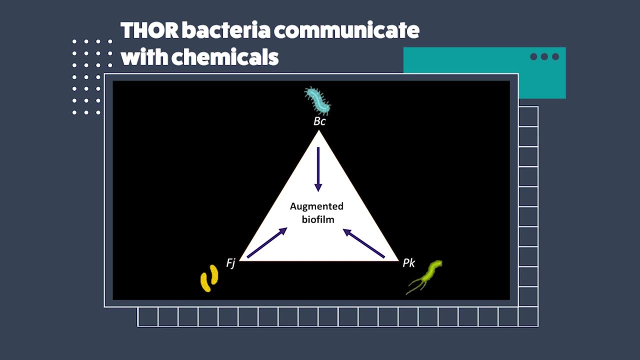 all of these different phenomena that I've shown you today. But what I would like you to remember is that these bacteria communicate with chemicals, like many other bacteria. So we've seen coriancins, which have certain effect on these different bacteria.